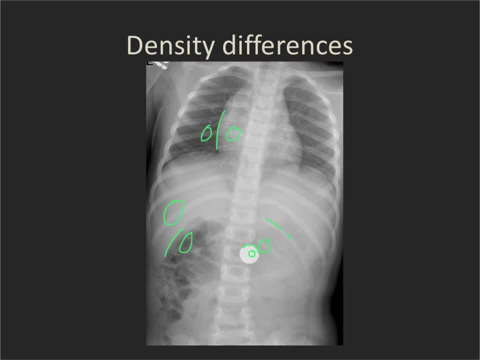 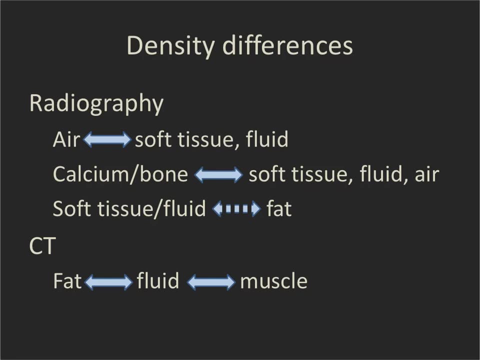 bi multiple tissue species, so it's in between the two In place of the two. So actually is didn't feel a rib because there's a difference between the calcific density of the rib and the overlying soft tissue. Now, with radiography, these density differences mean that we can easily see the 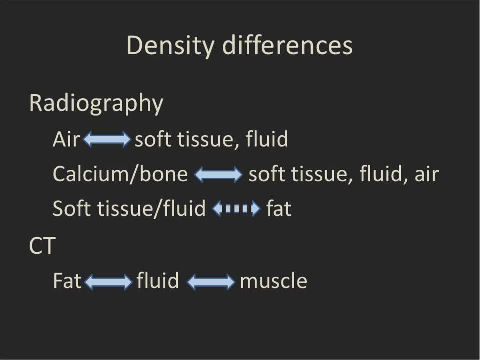 difference between air and soft tissue or fluid. We can see the differences between calcium and bone and soft tissue, fluid and air. However, we may not be able to see the differences between soft tissue or fluid and fat, because those density differences are much less and radiography is. 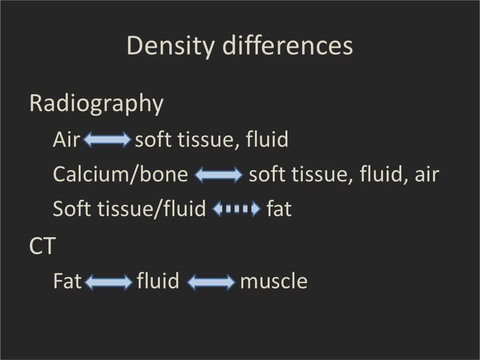 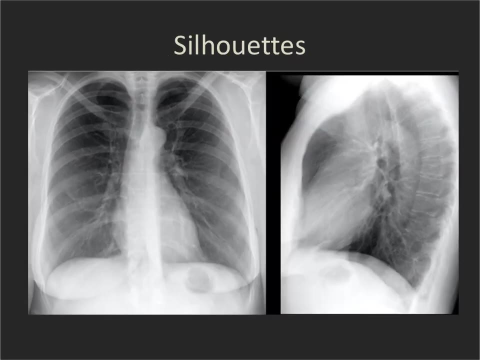 less sensitive to density differences than CT. With CT we're very sensitive to small differences in density and, depending how we window the images, we can easily see the differences between fat and fluid and muscle and even much more subtle density differences than that. So let's come back here to the term silhouettes. Where do we see silhouettes? on a chest? 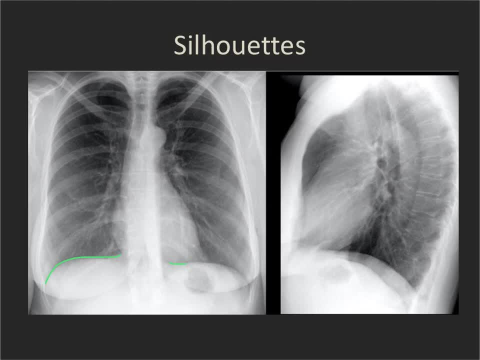 x-ray. Well, we see the silhouettes of both hemidiaphragms. We see those on both the frontal chest x-ray and the lateral chest x-ray. We see the silhouettes of the heart: the right heart border here, the left heart border here. We see the right side of the mediastinum. so this is the 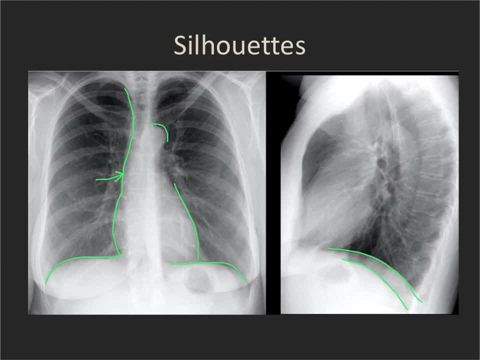 ascending aorta. there, for example, We see the aortic notch. We see the lateral side of the descending aorta On the lateral chest x-ray we see the lateral chest x-ray. On the lateral chest, the posterior aspect of the heart, We see the anterior aspect of the heart and the anterior. 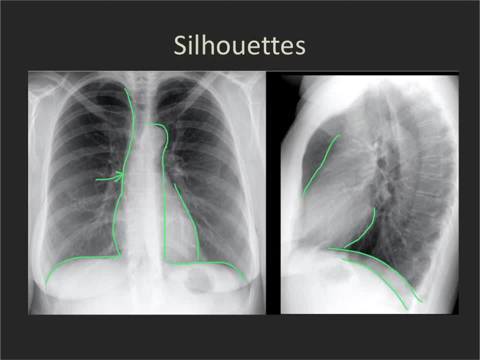 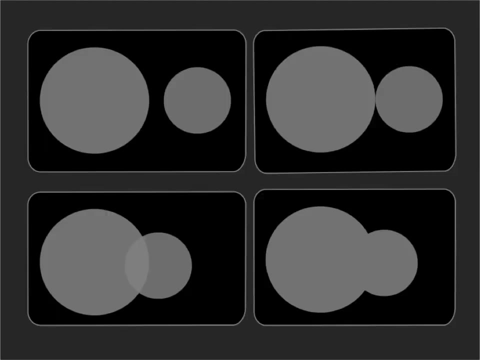 aspect of the ascending aorta. We can see the aorta, the posterior part of the posterior, most of the anterior border of the aorta throughout. So these are normal air soft tissue interfaces or normal silhouettes that we should be able to see. Now let's look at. 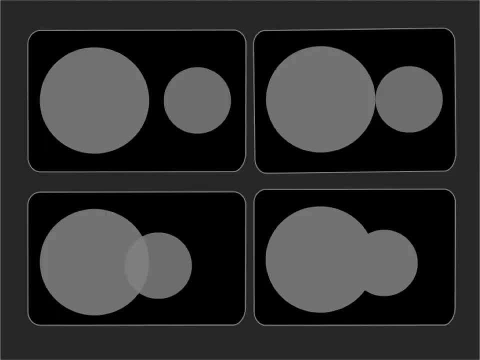 four hypothetical situations. So the gray circles here are objects and that's for illustrative purposes. Call this the mediastinum and this an area of pneumonia within the lung, And the black stuff here is all A. So in this example- here let's call this number one- we can see the silhouette. 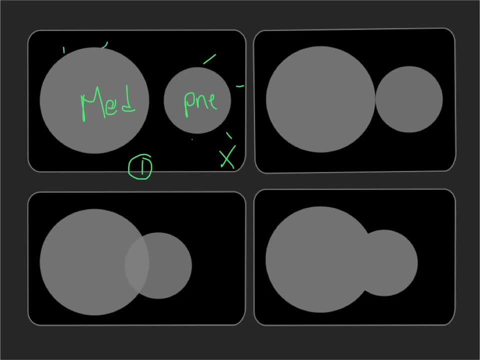 all the way around the pneumonia and, more importantly, we can see the silhouette all the way around the mediastinum Because there is no interruption of that normal air soft tissue interface. Now situation number two: the pneumonia is a little closer to the mediastinum, but it just 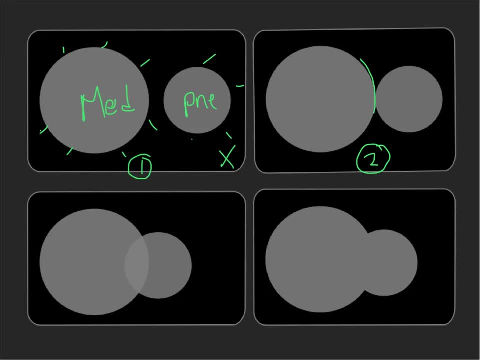 about touches it, but we can still see that normal silhouette of the mediastinum because it still has air all the way around it. Let's look at example number three Now. in example number three the pneumonia is behind The mediastinum. So it doesn't touch the mediastinum, but it's behind the mediastinum. So we can still see that normal silhouette of the mediastinum because there's still air up against it. 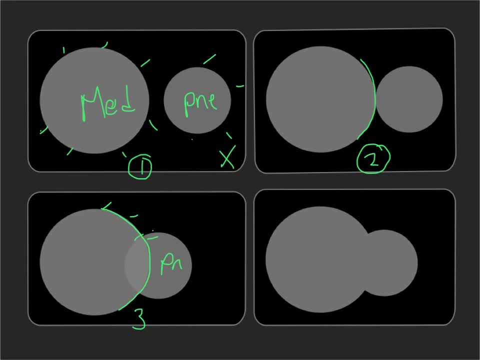 We can see the edge of the pneumonia at the back because it still has air up against it. And then there's this area in between that looks denser- so-called double density, because the x-rays are having to travel through two substances. Now, in example number four, that pneumonia here is right up against the mediastinum and there is no air between the pneumonia and the mediastinum. 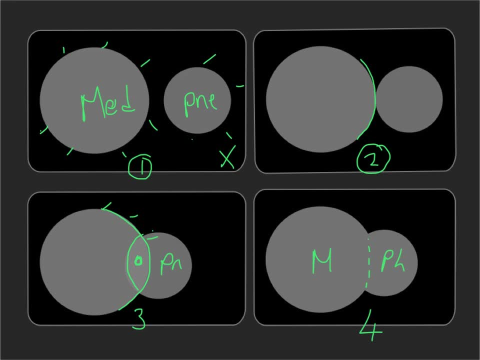 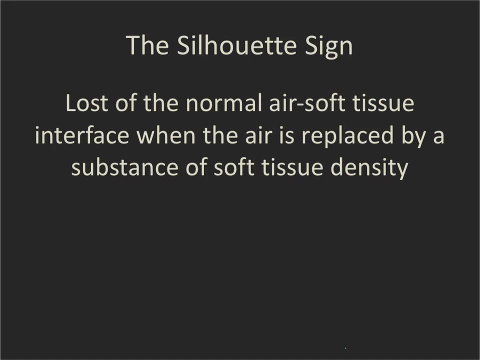 So you no longer have a silhouette and this is the silhouette sign. So the silhouette sign is the loss of the normal air soft tissue interface when the air has been replaced by something that is a soft tissue. It's the formation of comfortable tissue that the body, the air, complements. 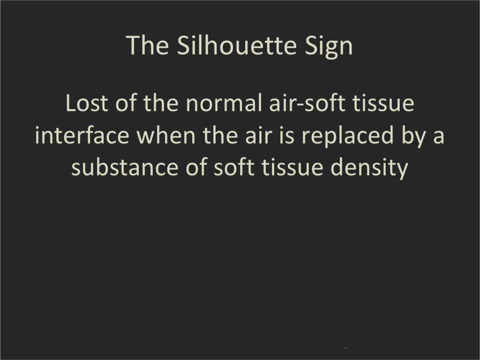 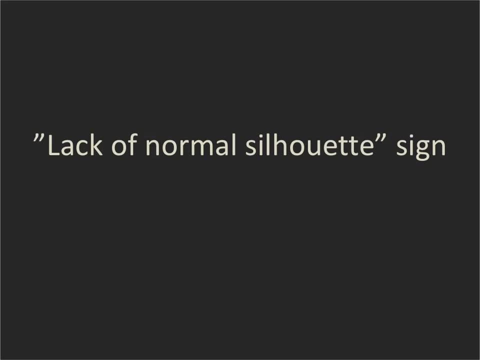 It's also the localized air that the ½ stuff gain the air, and the body plays a role in it staying good. So now you may ask you, what can I do with this Artemisia on this presentation? And we can do only one more application of this: ripeывайтесь, or at least as many of you as we can, right. 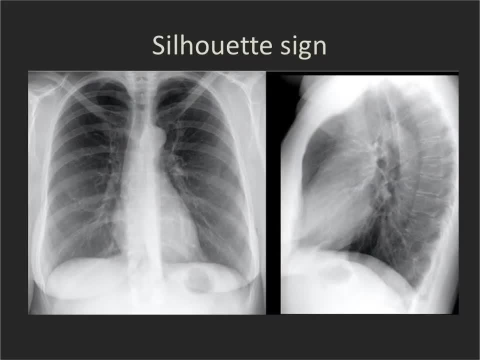 And that application would give you an idea as to why it's important to use melanoma Pneumonia or crystallite amputinatae Pneumonia. you can also Irritation, and I followed up on this appointment of this American. своего. 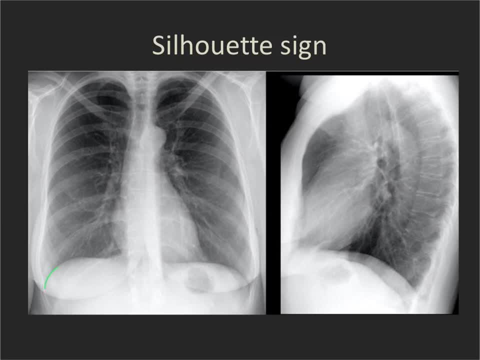 what lobe the abnormality is in. So if we lose the normal diaphragmatic silhouette on either side in either of the views, that is because of an abnormality in either the right lower lobe or the left lower lobe. If we lose the right heart border, that is because of something going on in the right middle lobe. 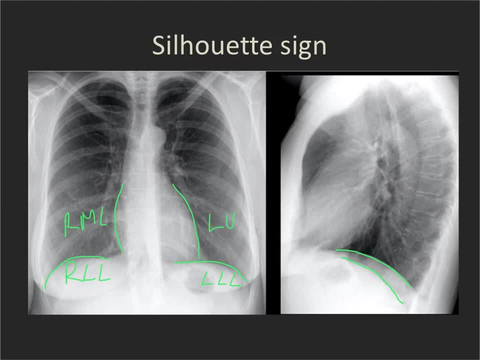 The left heart border. because of something going on in the left upper lobe, We lose the ascending aorta. that is the right upper lobe process. Same with up here into the right paratracheal area, The aortic notch, again that's a left upper lobe process. 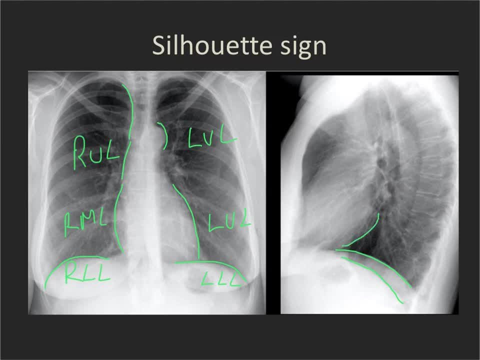 On the lateral chest X-ray. the posterior border of the heart is: if we have something going on in the left lower lobe, The ascending aorta here is because we have something going on in the left lower lobe, The ascending aorta here is because we have something going on in the right upper lobe. 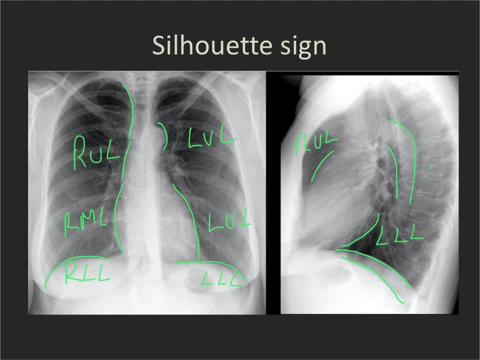 And the descending aorta, again because of a left lower lobe process. And that same left lower lobe process will make us lose that para-aortic line on the frontal chest X-ray. So seeing what silhouette you've lost is going to tell you what lobe the pathology is in. 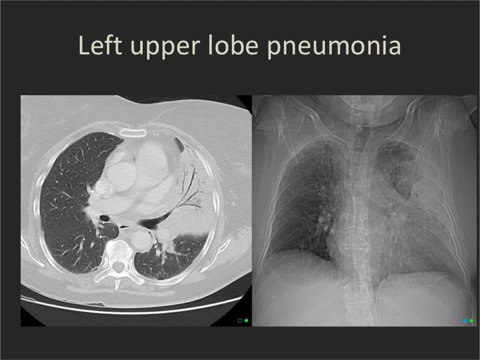 So let's just look at a couple of examples here. Here's a patient with a dense area of the heart. Here's a patient with a dense area of consolidation which was due to a pneumonia involving their left upper lobe. Let's look first of all at the CT scan here. 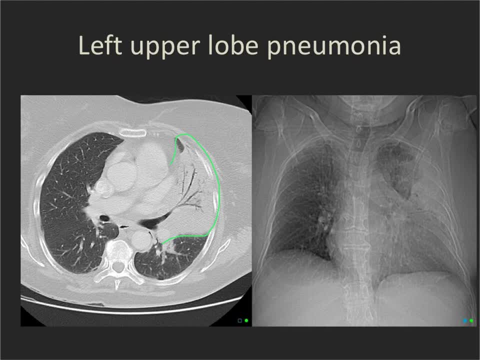 So we have this large area of consolidation. you can see some air bronchograms within it, in the left upper lobe, And you can see there is no air here between the left heart border and that area of consolidation, So we've lost the silhouette. 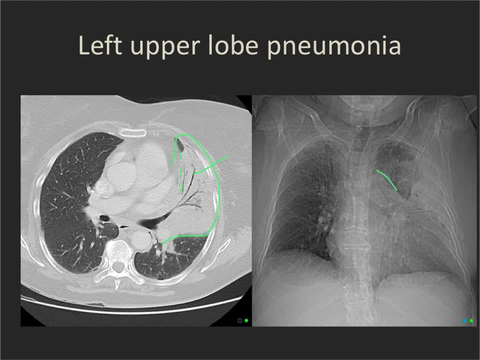 And this is shown here. This is the original. This is the original scan from the patient's CT scan, but it would look the same on a chest X-ray. Here's that area of opacity, And you can see here that we've lost the normal silhouette of the left heart border. 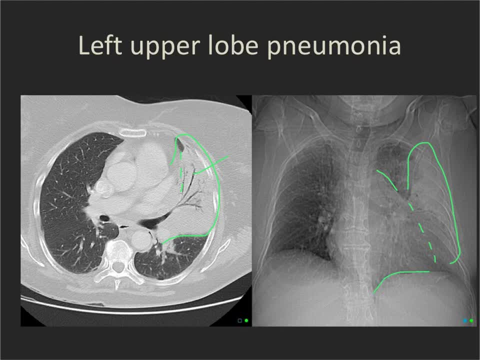 But notice how you're still seeing the left hemidiaphragm here. I'll just rub that out so that you can see it better. And that's because the left lower lobe, which abuts the left hemidiaphragm, is not involved.